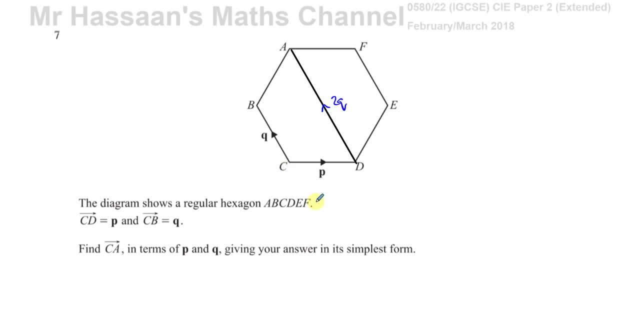 We could. I mean, I know that this is the vector 2Q basically. So I know from C to A is going to be the vector from C to D plus D to A. C to D plus D to A is the same as the vector from. 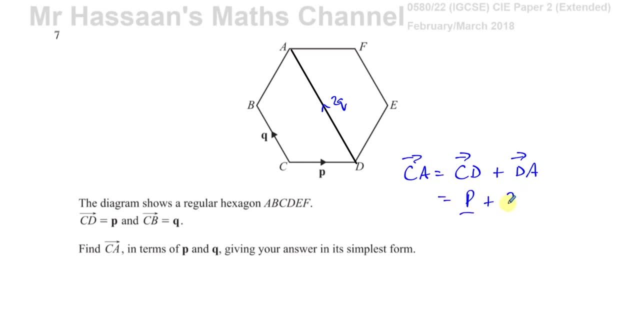 C to A, So that's going to be P plus 2Q, But why? I want to explain why in this question. Why is that the case? Now, if I were to take this hexagon and join the opposite corners, the opposite corners of each other, like this: 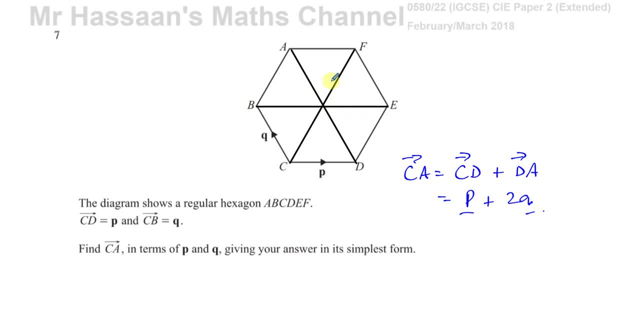 what I have formed here is basically a shape which has- Let me make it as accurate as we can- A shape which has A shape which has six triangles which are all the same. And how do I know that they're the same? Well, I know that in a regular hexagon, in a regular hexagon, if I was to extend one of the sides out, okay, 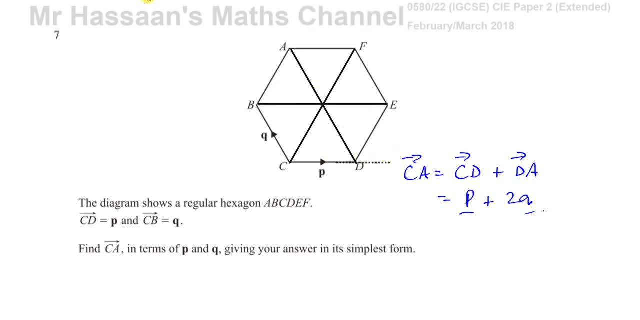 For example, if I was to extend this side out, I know that this angle here is going to be 360 divided by the number of sides, which is 60. So this angle here is 60 degrees. I know that And I also know that this whole angle 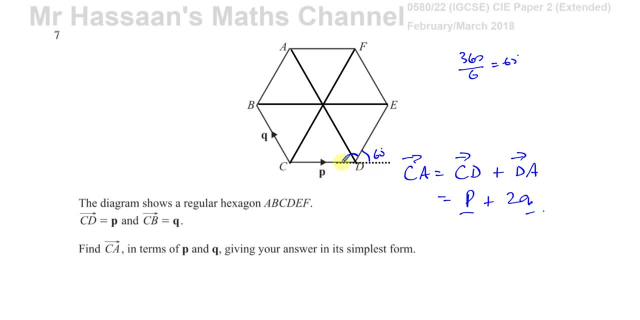 Inside. from there to there is 120 degrees, because they make like a straight line together this angle and that angle, because this is an exterior angle And if these two are, If this whole angle is 120, this is cutting this angle in half. so that's 60.. 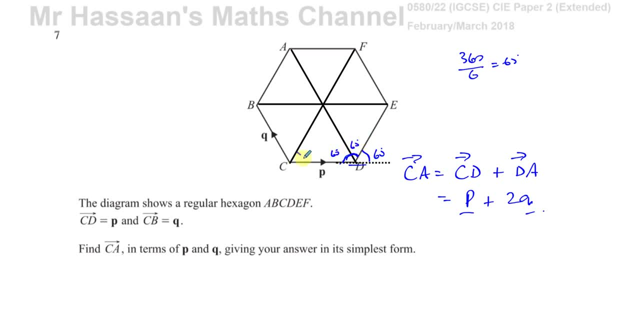 Therefore that's 60.. Okay, And that means it's the same in this corner, so that must be 60.. And also this, of course, has to be 60 as well. We've got: 360 divided by 6 is 60.. 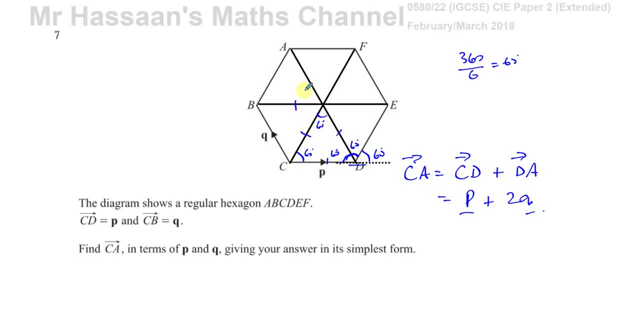 So basically, we have six equilateral triangles. These are all the same length. Okay, so we've got six equilateral triangles in here, And I know if this is 60 degrees, then this must also be 60 degrees, which means that these lines are parallel to each other. 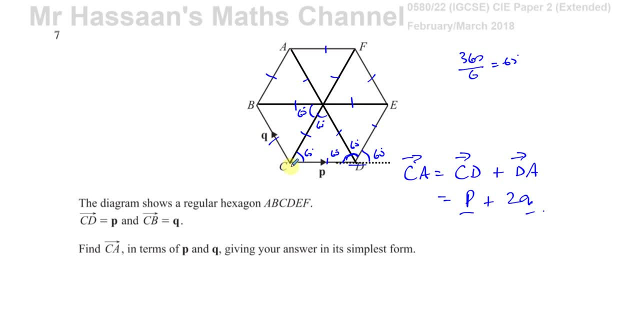 All right, These lines are all parallel. CD is parallel to BE, CB is parallel to DA. Okay, Because you know, if this angle is 60,, all right, And if I know also that this angle is also 60,, okay. 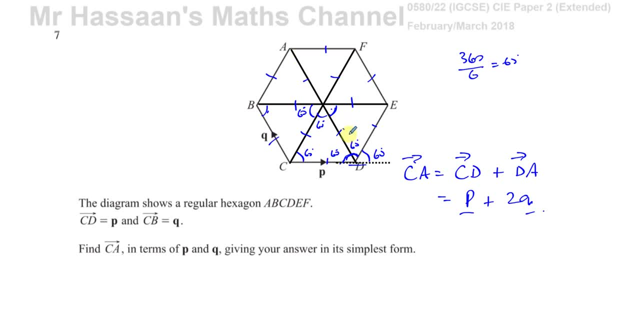 Then this Line is parallel to that line because I make an F-shape. So if these two lines are parallel, they can be expressed in terms of the same vector And I know that this is the same length as Q And it's parallel to Q. 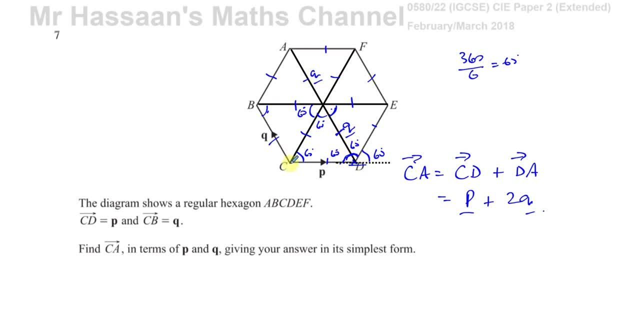 So this is Q and this is Q, So this gives us 2Q. So, to go from C to A, you're going to have P plus 2Q, All right, So because each of these are equilateral triangles, all these lengths are the same. 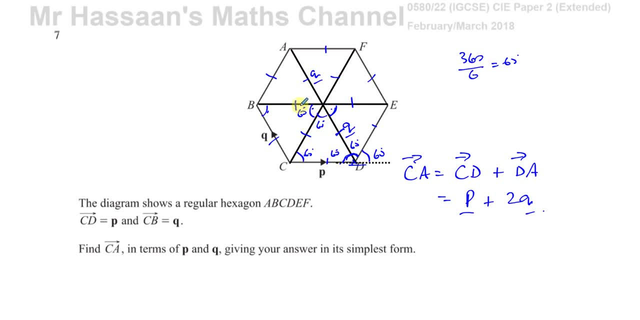 And because these are equilateral triangles, this angle is equal to that angle. So this and this line are parallel. This and this line are parallel, These lines that are going across like this: they're parallel to each other, That line is parallel to that line, and so on. 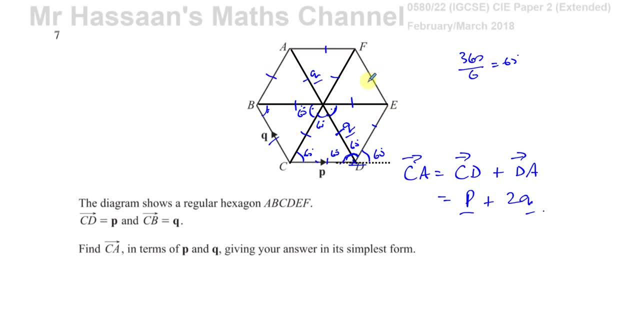 These opposite sides are parallel to each other, So that could also be considered vector Q as well. All right, So for that reason, I'm going to get rid of all of this now to make it look neater. So for that, that's the reasoning behind it. 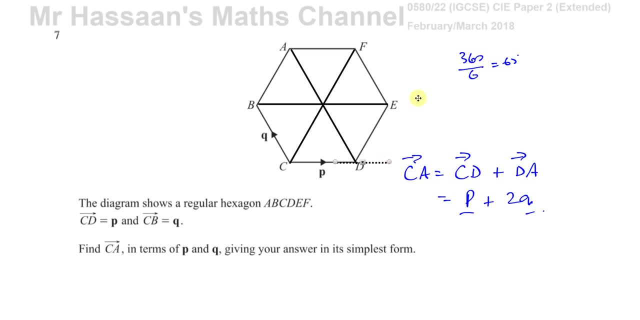 You don't have to prove it here at all. Okay, If you just quote the fact now that the vector D to A is 2 times Q, that's fine. But I just showed you the reason, Because this is Q and this is Q. 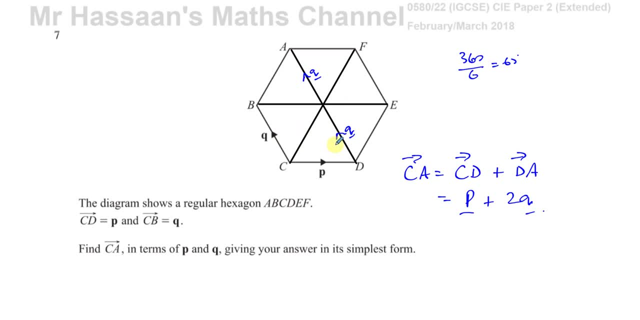 Because of these six equilateral triangles, this length is the same as that length And this line is parallel to that line. Okay, This line, because this angle is 6D, as is this angle, So therefore this makes an F shape, basically. 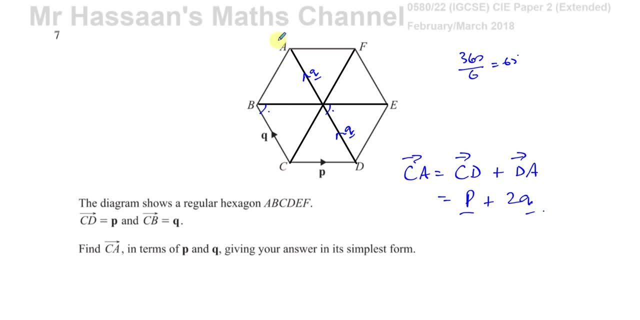 So this is the angle. I'm sorry, This is the vector from C to A. It's like going from C to D plus D to A, So all questions involving these type of regular hexagons Vectors can be solved using this idea. 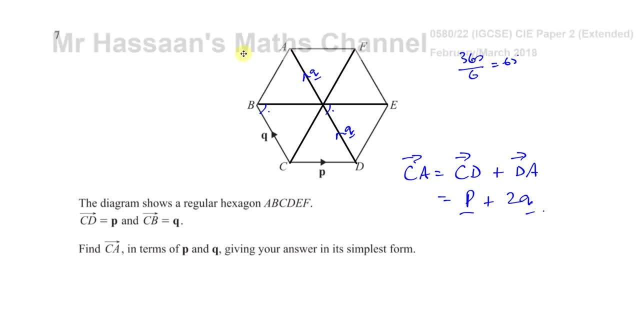 Okay, So these lines weren't there in the beginning. In the beginning, we didn't have any of these lines. Okay, None of them were there. In the beginning it looked like this, But I know, because of what I just mentioned, that this line, okay, is the vector 2Q. 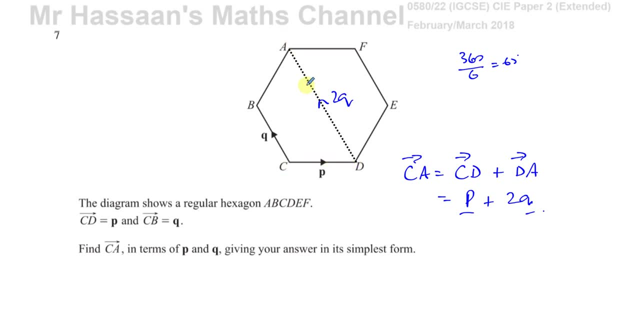 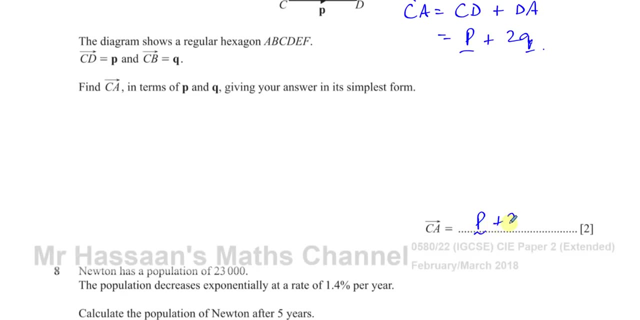 So this is C D, P, D, A, 2Q, P plus 2Q. Okay, So that's the answer So to this question: P plus 2Q. That's a very simple way of answering this question. 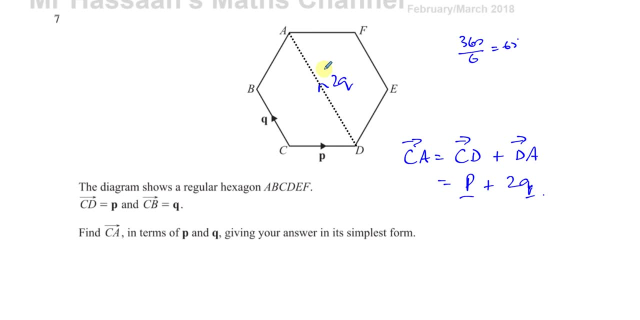 You don't have to prove it, You can show it, You can just quote it. Okay, You have to understand that. that's one of the properties of a regular hexagon: that the opposite, the sides which are going across like this, are all parallel to each other.